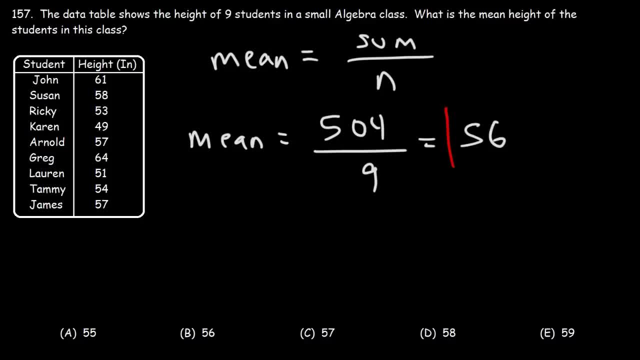 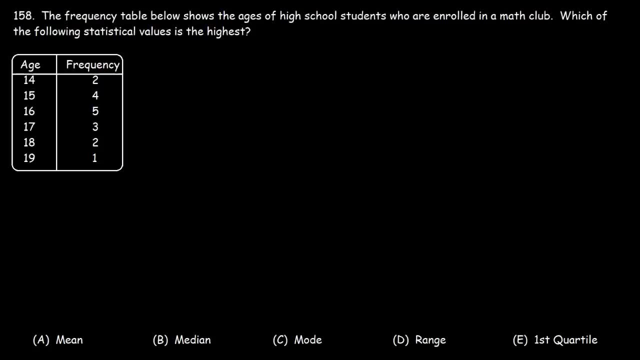 56.. So this is the average height, or the mean height of all the students in this class. B is the answer Number 158.. The frequency table below shows the ages of high school students who are enrolled in a math club. Which of the following statistical values: 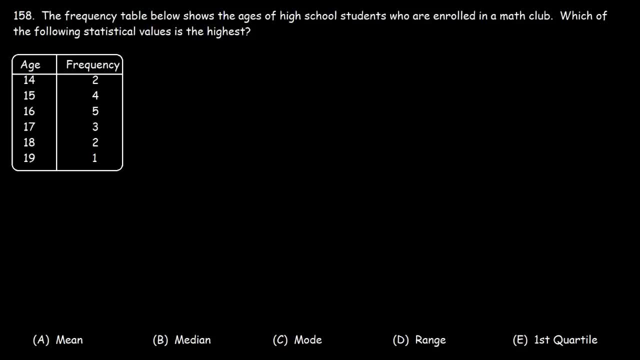 is the highest? Would you say it's A- the mean, B the median, C- the mode, Or would you say it's the range or the first quartile? Let's calculate each value. Let's start with the first one, the mean. So we said that the mean is equal to. 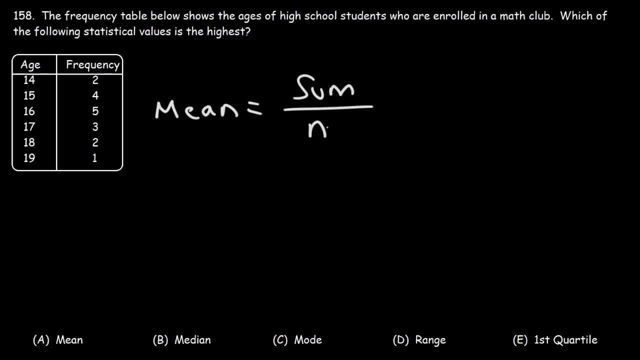 the sum divided by the number of items in our list. Now what we have is a frequency table. In order to calculate the mean of a frequency table, you need to take the sum of the numbers, Number 159.. The frequency table below shows the ages of high school students who are enrolled. in a math club. Which of the following statistical values is the highest: B- the median. B- the median. Which of the following statistical values: B- the median C the median A the median B. the median C. the median B. the median C. the median B. the median. 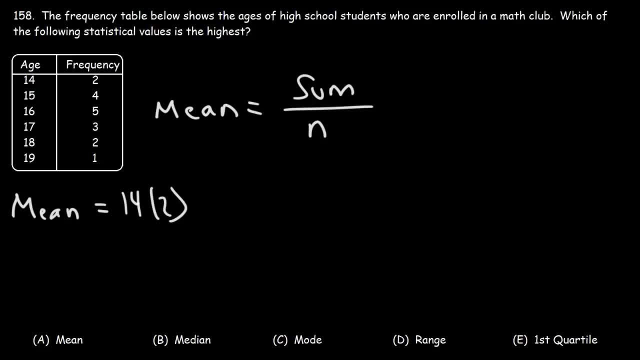 And of the following statistical values should be calculated. Number one: The human age is 14 years old, So the sum of their ages is 14 plus 14, or simply 14 times 2.. There's four students who are 15 years old, So the sum of their 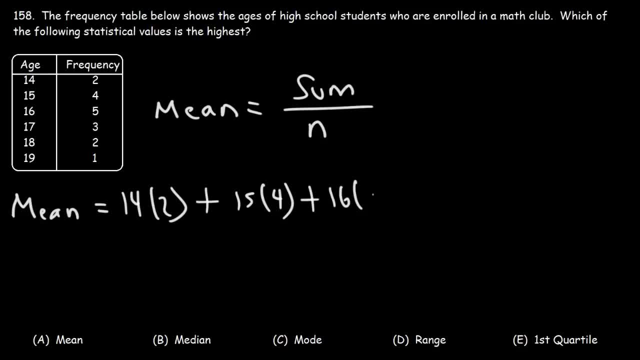 ages will be 15 times 4.. And then just follow the pattern. Next is 16 times 5, and then 17 times 3,, plus 18 times 2,, plus 19 times 1.. Now we'll need to divide it by whatever. 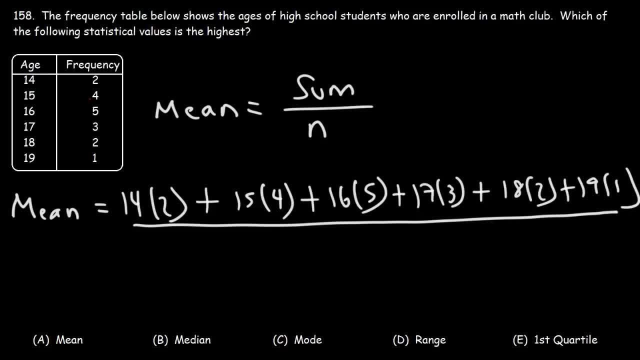 number we have Number one: The average height is the most common number in a math club. It's about the total number of students in this club, which is the sum of the frequency column. so we have 2 plus 4, which is 6 plus 5, that's 11, then 14, 16, 17.. so there's a total of 17 students in this club. 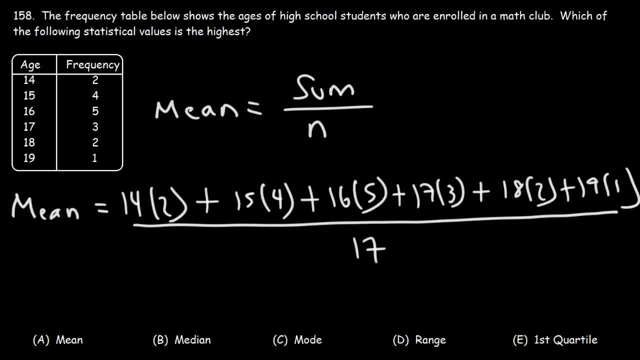 go ahead and type this in your calculator, so you should get, for the mean, 16.118. now let's do the same for Part B. let's calculate the median of this group frequency table. so how can we do this? the best thing we could do right now is write out the numbers. 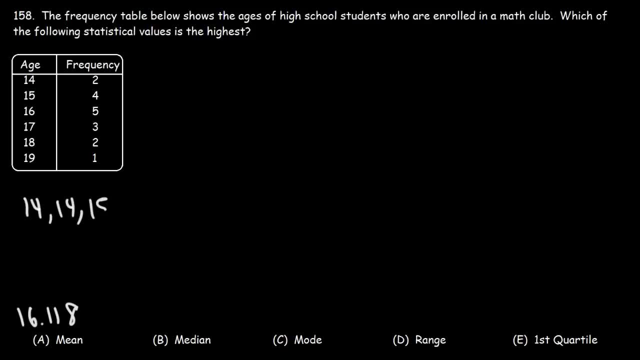 so we have 214, four fifteens- You want to write this in increasing order- And then we have five numbers with a value of sixteen, three seventeens, two eighteens, one nineteen. The median is basically the middle number. So we're going to eliminate numbers on the left. 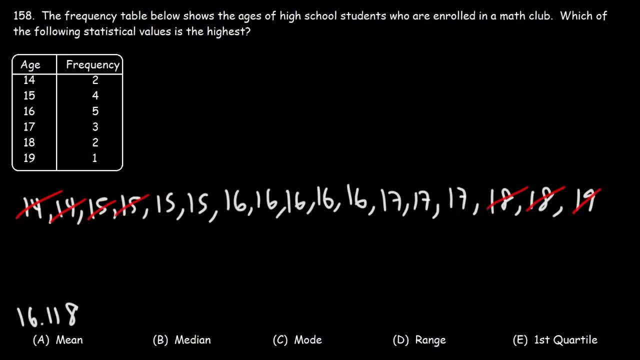 side and on the right side, until we find what number is in the middle. So we can see that the median is sixteen in this example. Now what about the mode? The mode is the number that occurs most frequently. The number with the highest frequency is sixteen. so that's the mode. The range is the difference. 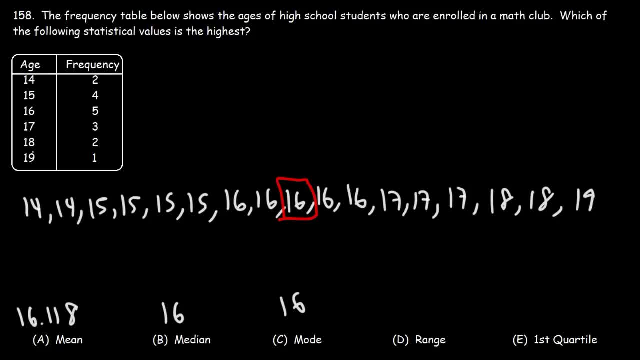 between the highest number and the lowest number. The highest number is nineteen, the lowest number is fourteen. So the range is going to be nineteen minus fourteen, which is five. Now what about the first quartile? The median represents the second quartile. To find the first quartile, you need to 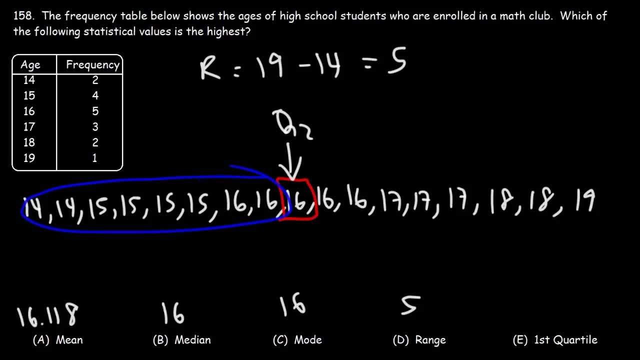 find the median of the lower half of the data. So what is the median of those first eight numbers? The median is going to be fifteen, So fifteen is the value of the first quartile. So the answer for this problem is answer choice A. The mean is the. 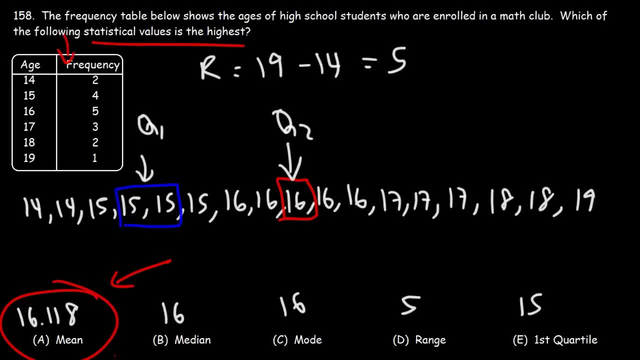 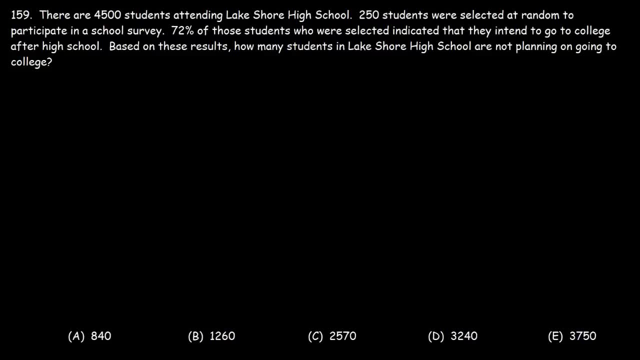 highest statistical value based on this frequency table Number 159.. There are 4,500 students attending Lakeshore High School. 250 students were selected at random to participate in the school survey. Seventy-two percent of those students who were selected indicated that they intend to go to college after high school. Based on these results, 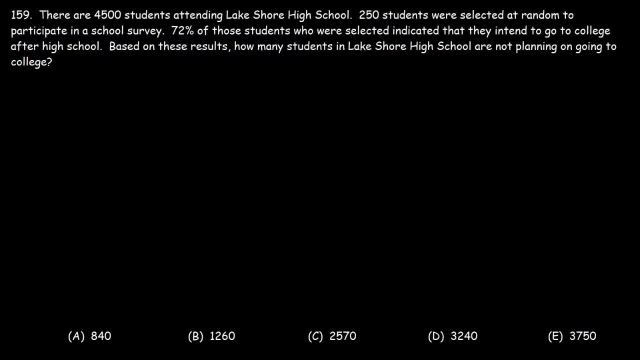 and the numbers shown here. a young man completed at least 20 years of assessment before graduating. This depends on the age of the young. How many students in Lakeshore High School are not planning on going to college? Let's write down what we know. Seventy two percent of students who participated in a survey say aquele. 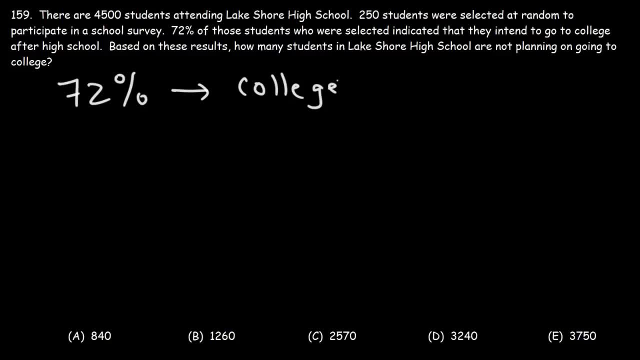 they want to go to college. That means that the other twenty-eight percent are not planning on going to college. A hundred minus seventy-two is the average amount of time a student is limited to. sipping is 28.. So, in order to answer this question, in order to determine the number of students in the 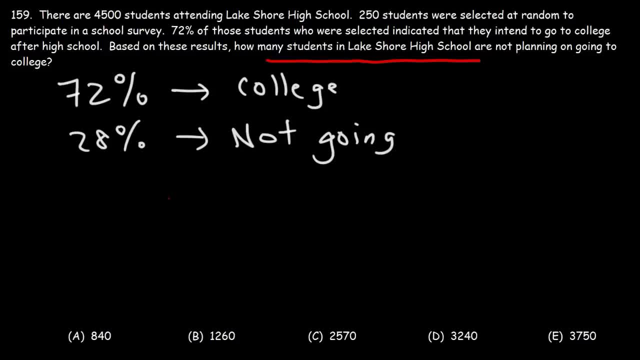 entire Lakeshore High School who are not going to college. we simply need to find 28% of that number. So what is 28% of 4,500?? All we need to do is take the decimal equivalent of 28%. 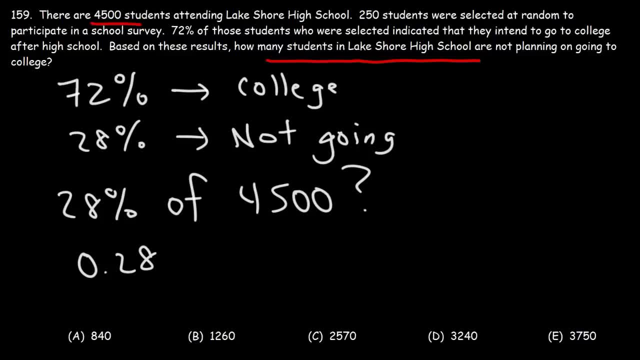 which is 0.28, just take 28% divided by 100, and then take that number, 0.28, multiply it by 4,500. You should get 1,260.. So that's the number of students who are not planning on going to college. 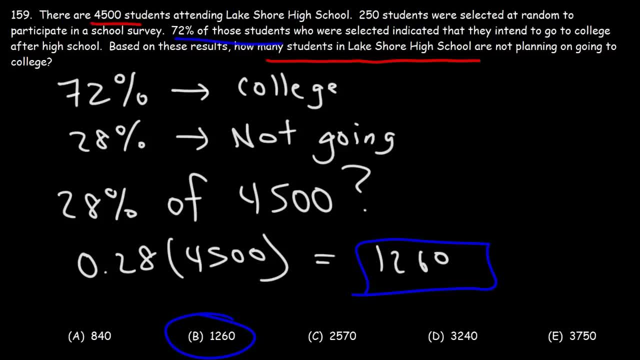 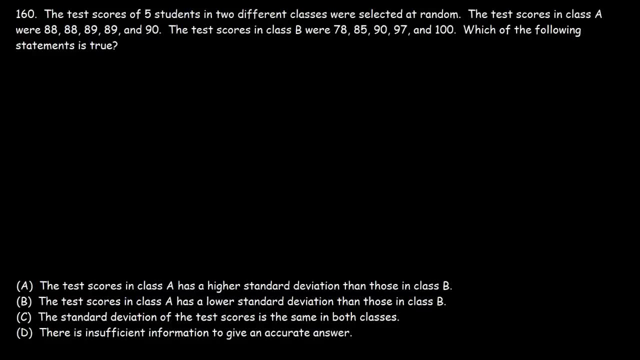 based on the data that we've got received from this survey Number 160.. The test scores of five students in two different classes were selected at random. The test scores in class A were 89, I mean 88,, 88,, 89,, 89, and 90.. 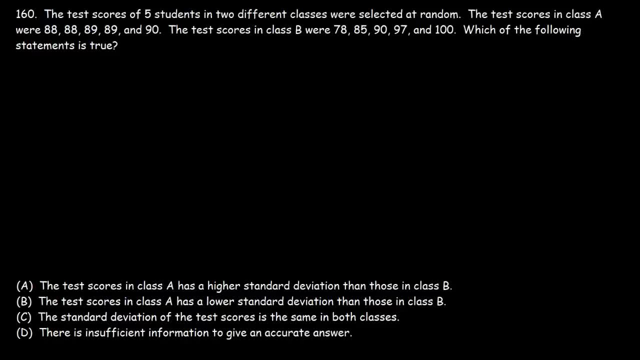 The test scores in class B were 78,, 85,, 90,, 97, and 100.. Which of the following statements is true? So let's look at answer choice A: The test scores in class A has a higher standard deviation than those in class B. 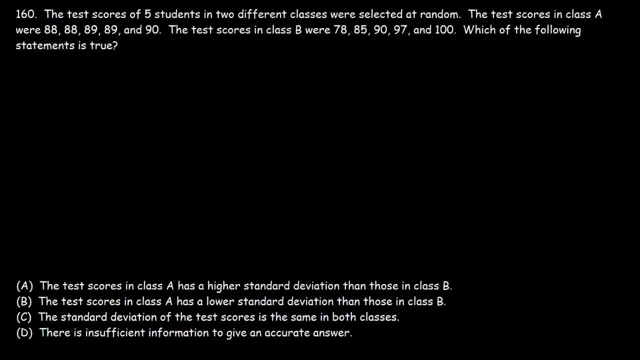 Is that true or false, Or is it the other way around? The test scores in class A: does it have a lower standard deviation than those in class B, Or are the standard deviations the same for the two groups? Well, let's write out the data in such a way that will help us to answer the question. 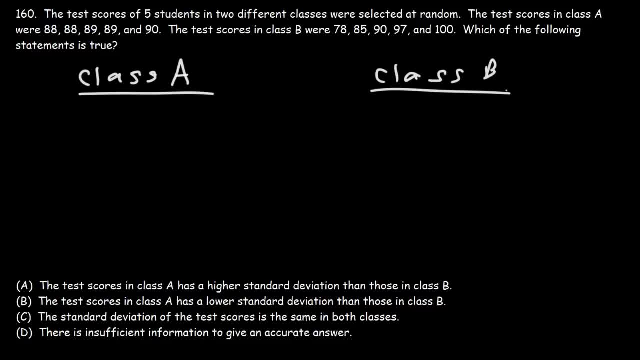 The standard deviation tells us how far the data set values are from the mean. In class A we have the scores 88,, 89,, 90, 89, and 88. If you average these five numbers, you'll find that the data set values are from the mean. 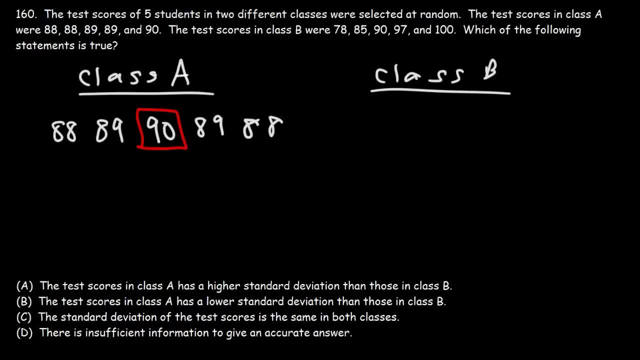 The mean is 90.. It's the number right in the middle Class. B have the scores 78,, 85,, 90,, 97, and 100. If you add up those five values and divide them by five, you'll find that the mean is also 90.. 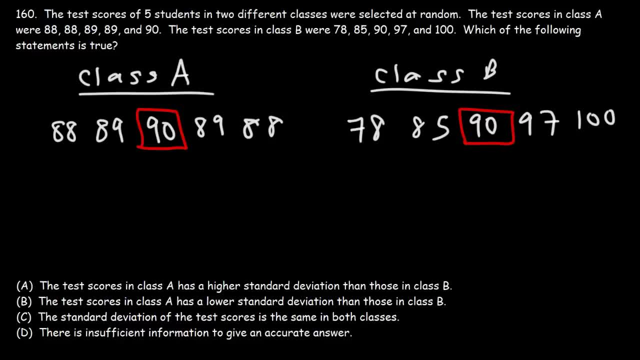 Now let's give consideration to how the numbers are arranged and how they relate to the mean. So, looking at these two classes, which one has a higher standard deviation with respect to their test scores? Is it class A or is it class B? Now, keep in mind: the standard deviation tells us how far the data values are from the mean. 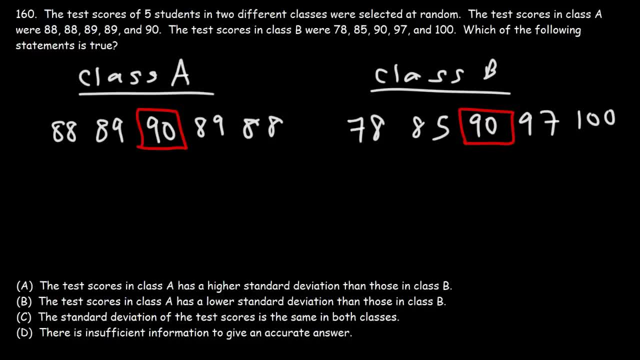 So which class has a higher standard deviation? This class has data values that are very close to the mean. That's class A. All the test scores are very close to 90, which is the mean. So therefore, class A is going to have the lower standard deviation. 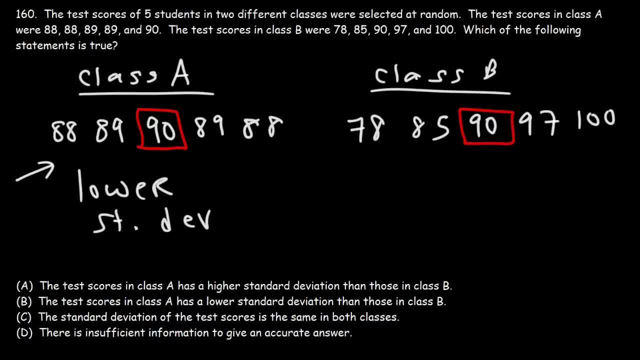 Class B, on the other hand, has test scores that are very far from the mean. Therefore, it's going to have a higher standard deviation. So the correct answer for this problem is going to be answer choice B. The test scores in class A has a lower standard deviation than those in class B. 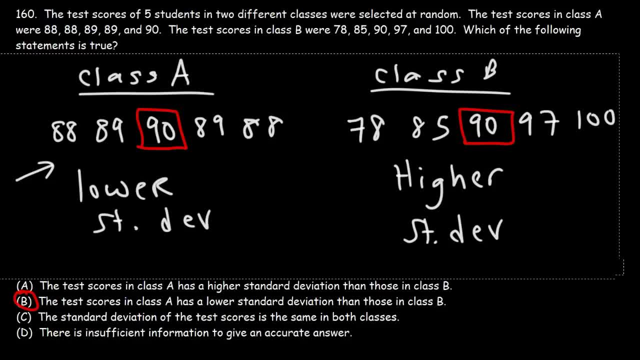 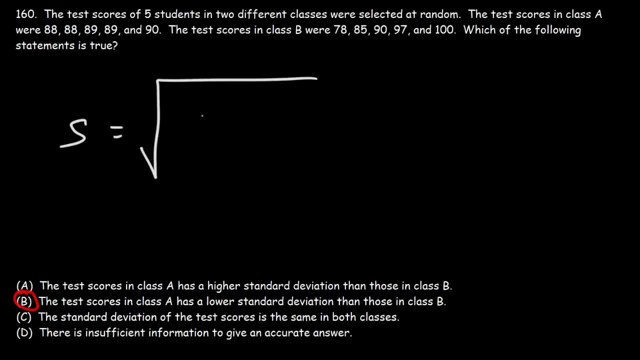 Now, for those of you who would like to verify this, here's the formula that will help you to calculate the standard deviation. The standard deviation is the square root of the sum of the square differences between all of the data values and the mean divided by n-1.. 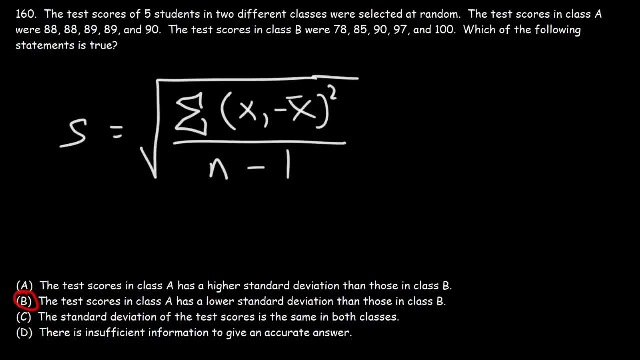 So you could use that formula to see which group has the higher standard deviation. 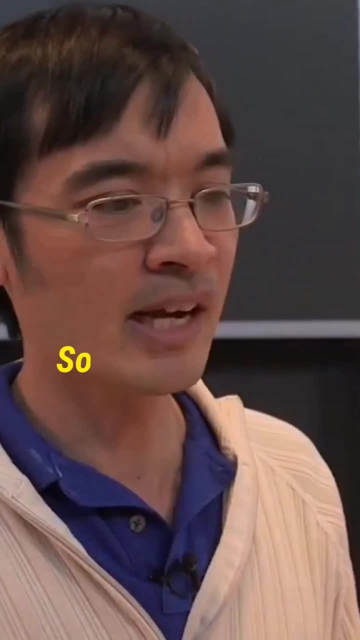 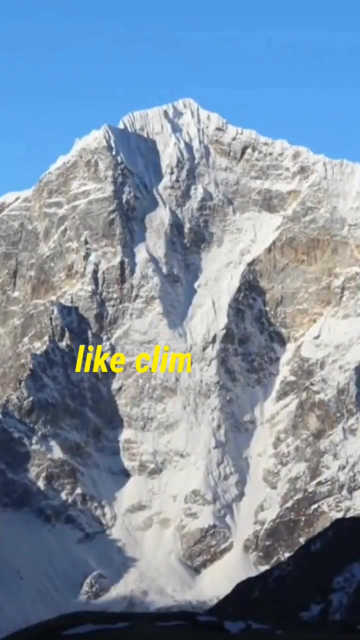 You know you can't really call your shots in mathematics. Sometimes the tools are not there. It doesn't matter how smart or quick you are. The analogy I have is like climbing: If you want to climb a cliff. that's 10 meters high. 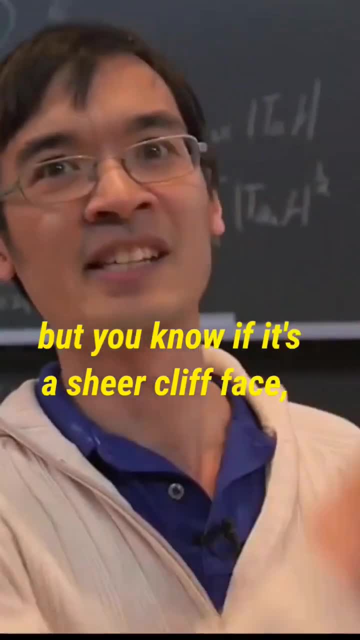 you can probably do it with the right tools and equipment. but if it's just a sheer cliff, face you know, a mile high and there's just no handholds whatsoever. you know, just forget it. It doesn't matter how strong you are or whatever. 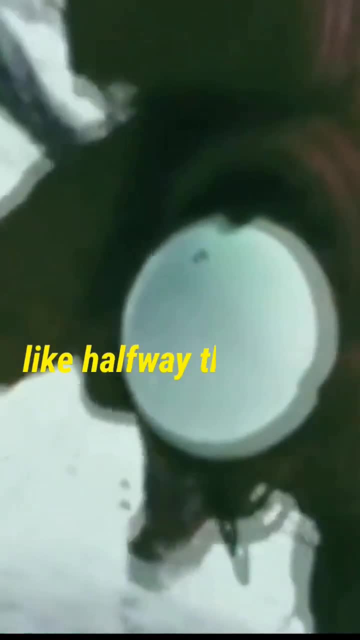 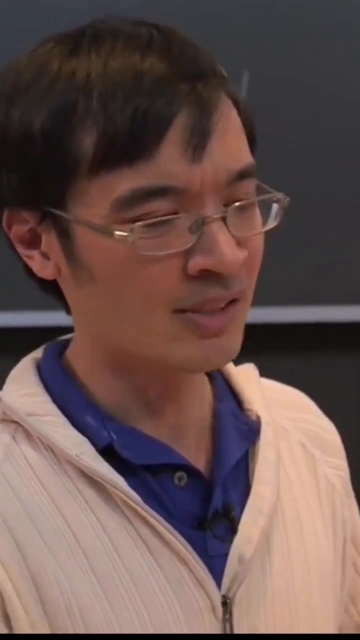 You have to wait until there's some sort of breakthrough, like some opening occurs, like halfway through, halfway up the cliff, and now you have some easier sub-goal. You know there are some speculations. There's some possible ways to attack the conjecture. but nothing is really promising currently. 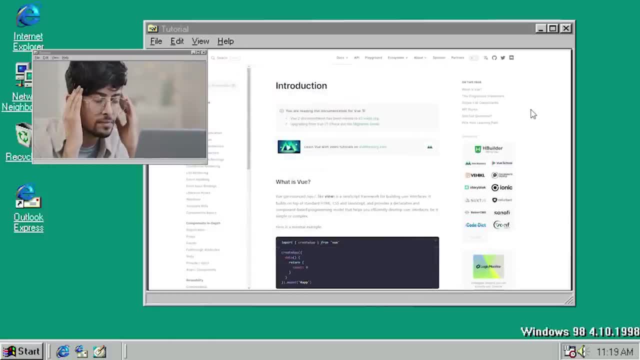 Well, let me make it a little easier for you. While React has the benefit of name recognition, there are other frameworks that, 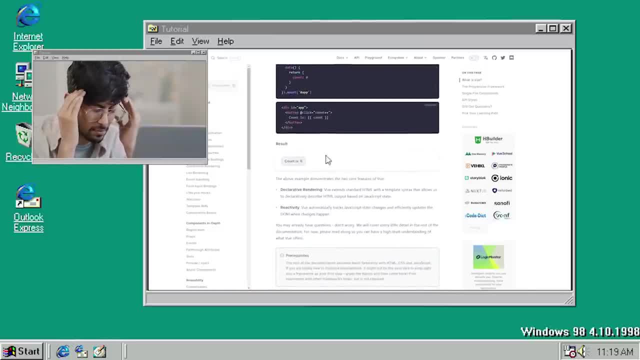 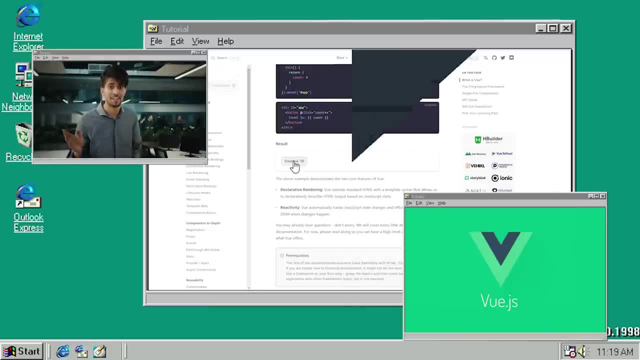 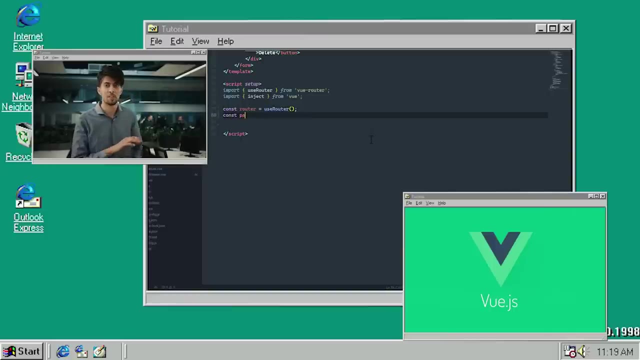 in my humble opinion, do a much better job. For example, Vue.js is extremely approachable if you already know a little HTML, CSS, and JavaScript. Its feature set is easier to understand and use. It's very, very fast and its growing community is ready to jump in and help if you have any questions. 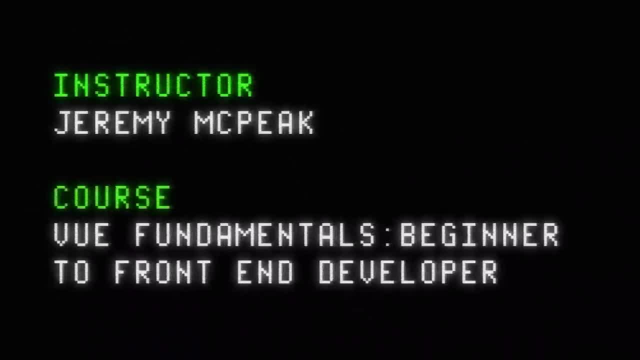 Hi, I am Jeremy McPeak and I'd like to teach you everything that you need to get started with Vue.js.